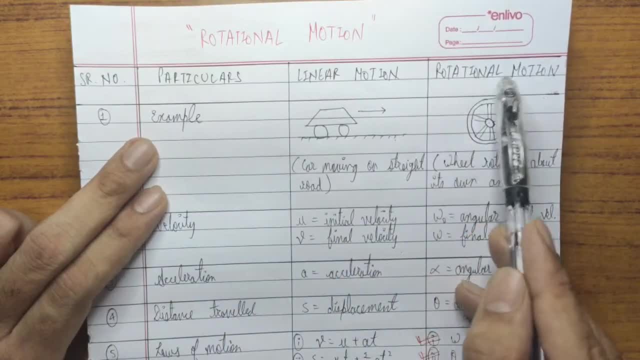 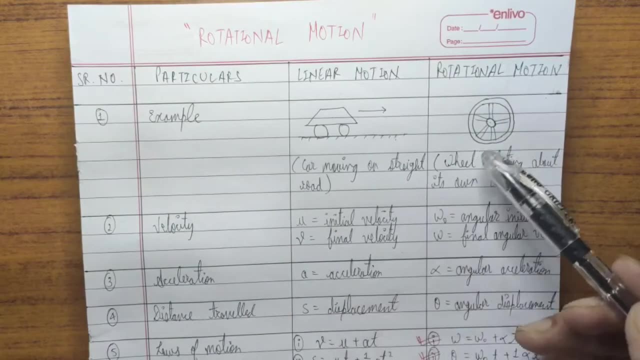 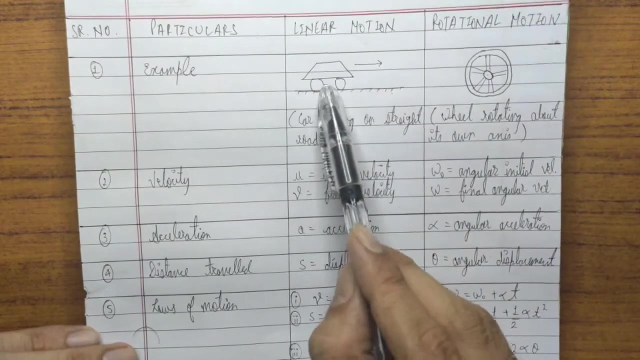 So I hope you have understood what is linear motion and rotational motion by considering the example first. Now we will go into detail about the various formulas which are used in both the motions. When this car is moving on a straight road, it is covering a certain distance, So there is displacement involved. 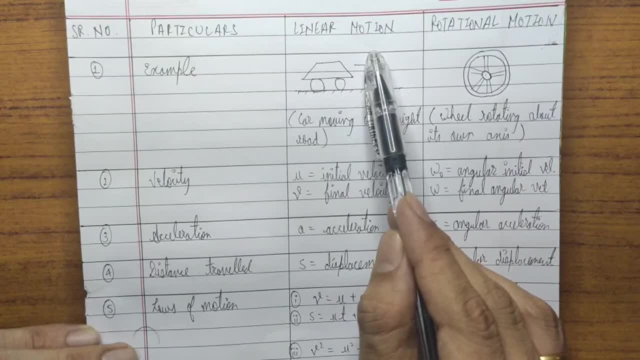 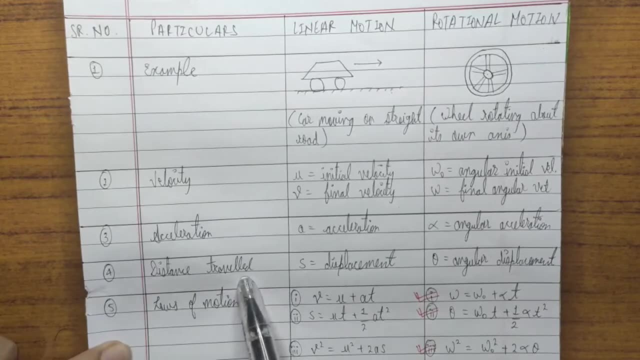 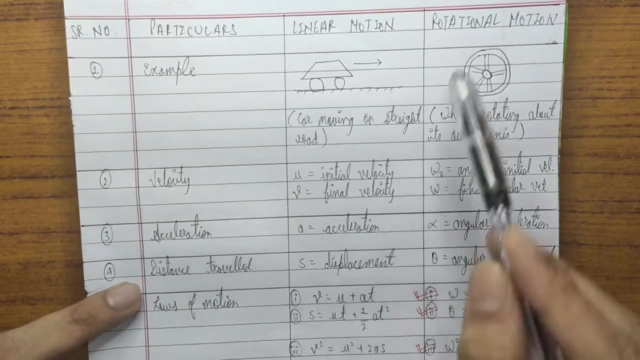 And in linear motion, we know, the displacement is represented by S. So the distance travelled by the car is nothing but the displacement, and it is represented by S. And in rotational motion the displacement is represented by theta, And that displacement is an angle. 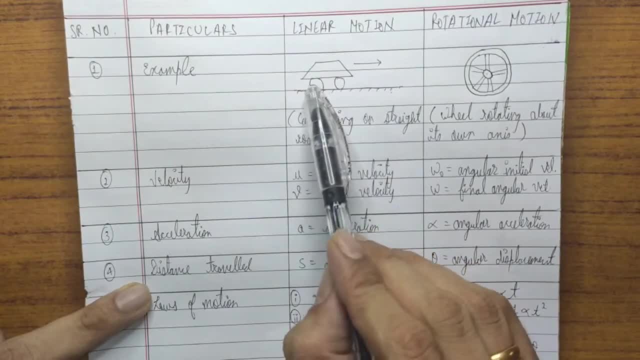 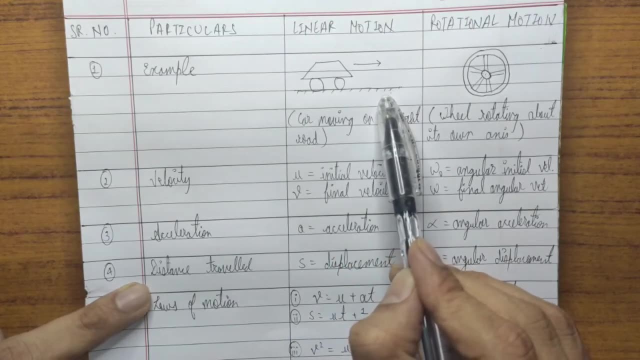 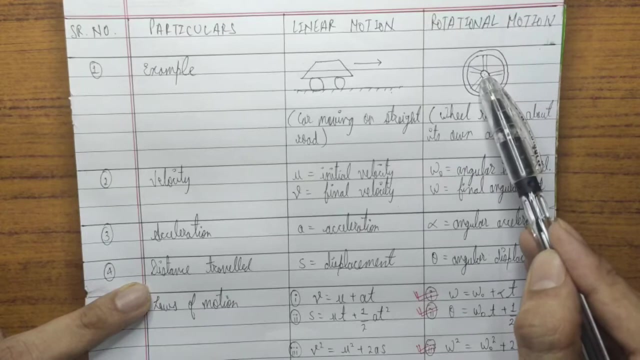 See, here the car is moving on a straight path, So the distance covered will be linear distance. that may be expressed in meters. But in this case what is rotational motion? Rotational motion is the motion of the wheel about its own axis. So about its own axis, the wheel will rotate at same position by a certain angle. 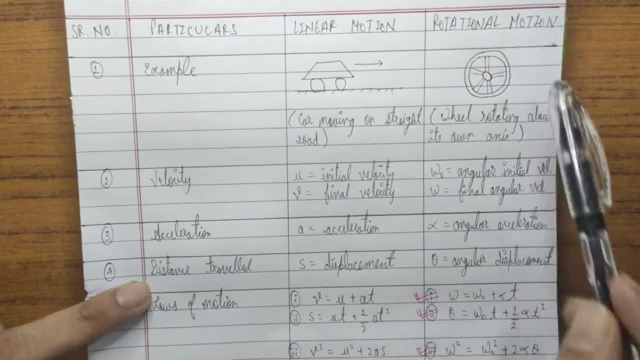 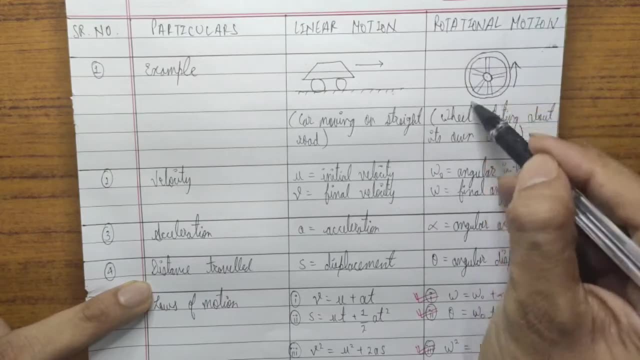 So displacement in this case will be in terms of angles. This particular wheel is rotating around its own axis. This particular wheel is rotating in, say suppose, anti-clockwise direction, Suppose in this direction. So the displacement of this wheel will not be linear. 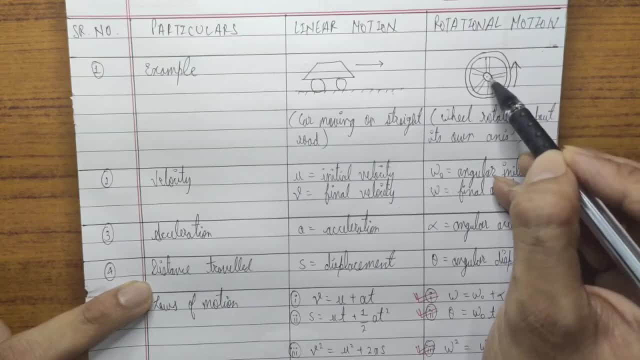 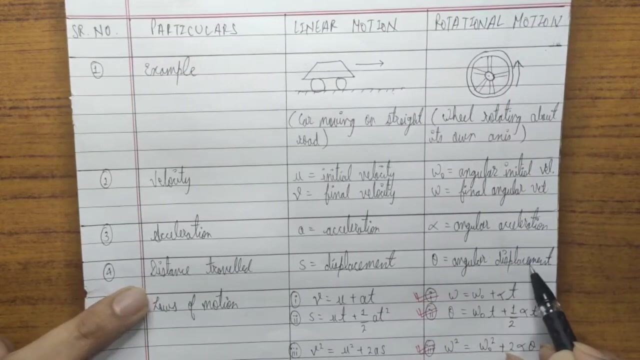 It is not moving from this place to this place. At the same place, it is rotating or it is displacing. The displacement of the wheel is in terms of angle And that angle is angular displacement. The displacement is known as angular displacement. 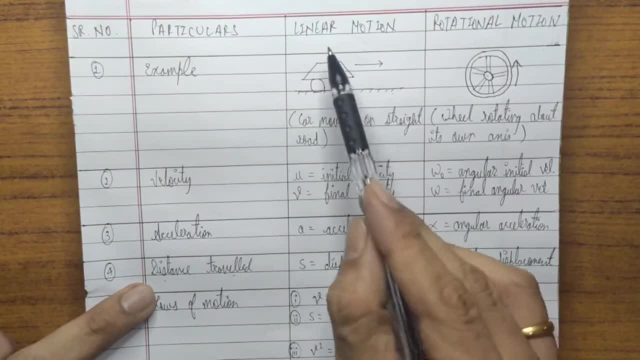 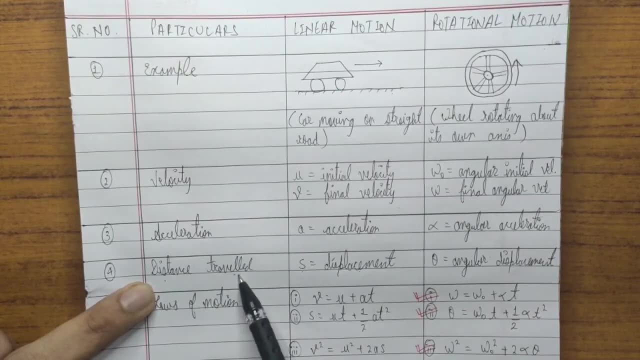 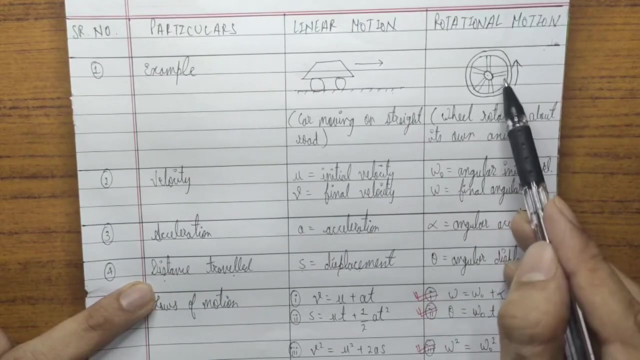 So the distance travelled in terms of linear motion. In terms of linear motion, is known as displacement And it is represented by S. However, distance travelled in rotational motion is represented by theta And it is known as angular displacement. So in this case, there is angular displacement. 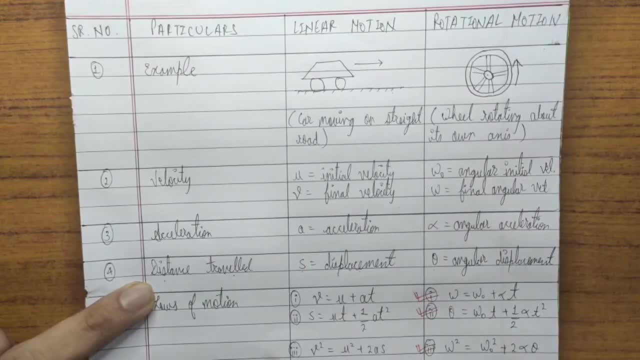 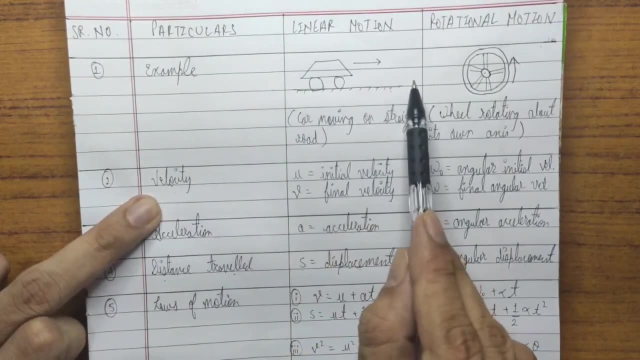 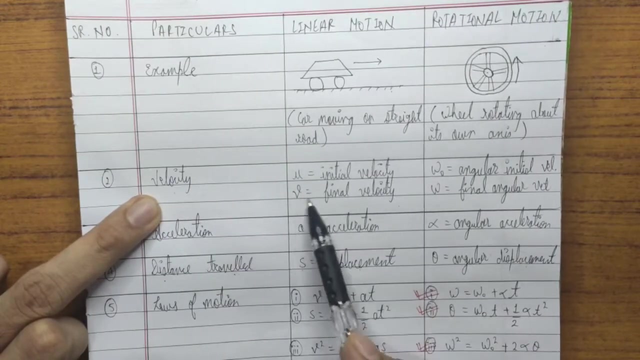 And in this case there is a linear displacement. Now, since in this case there is a linear displacement, So the velocity will be linear velocity. And in velocity we have studied two types of velocity: U and V. U was the initial velocity and V was the final velocity. 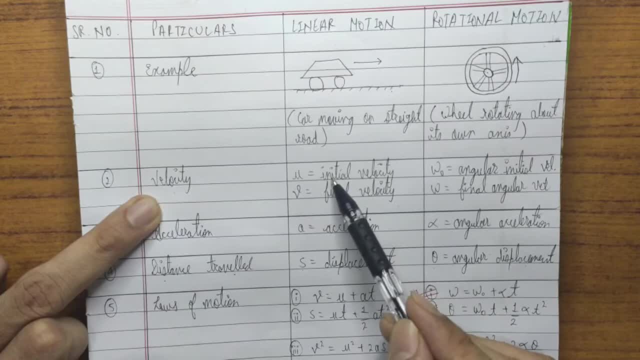 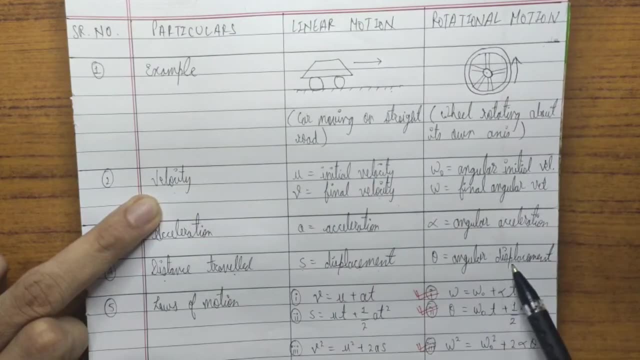 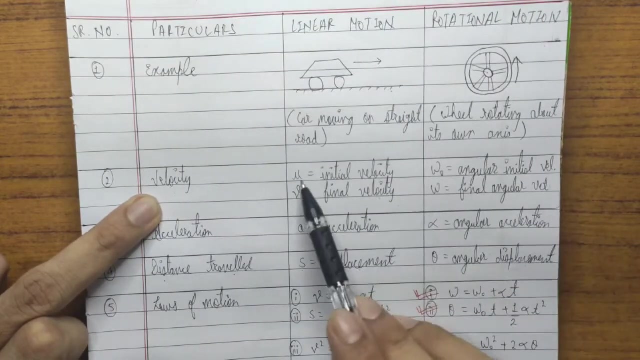 So, since there is a linear displacement, So there is linear initial velocity and linear final velocity. Why? Because the displacement is linear, But in this case the displacement is angular, So the velocity will be angular velocities. So here it is represented by U, which is initial velocity. 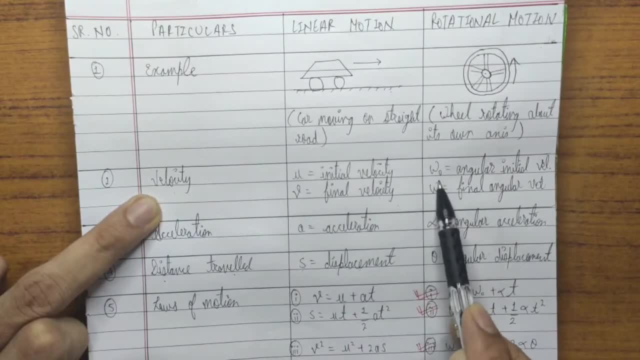 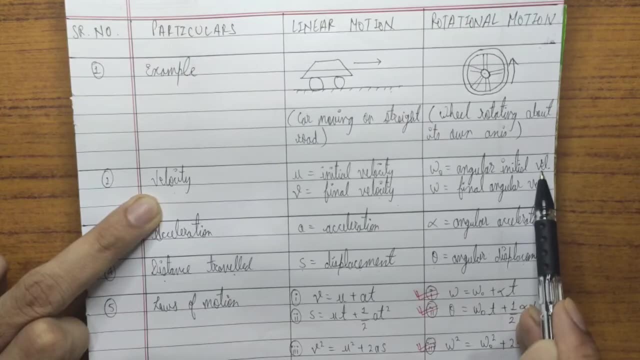 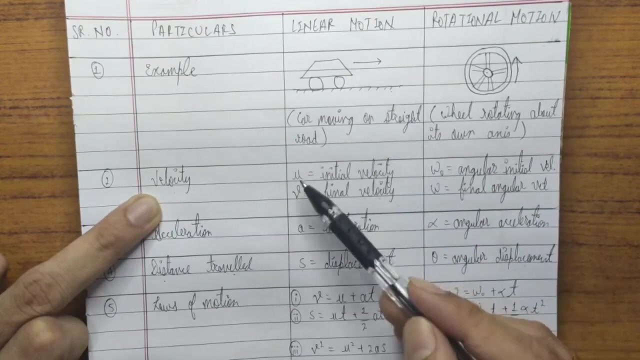 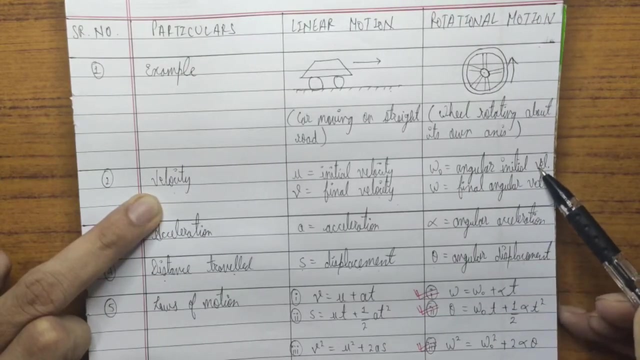 So in rotational motion u is replaced by omega not, okay. or you can write omega zero. it is angular, initial velocity, okay, it is velocity, but it is angular and it is initial, okay. so in linear motion there is initial and final velocities. in rotational motion there is omega not, which is initial angular velocity, and 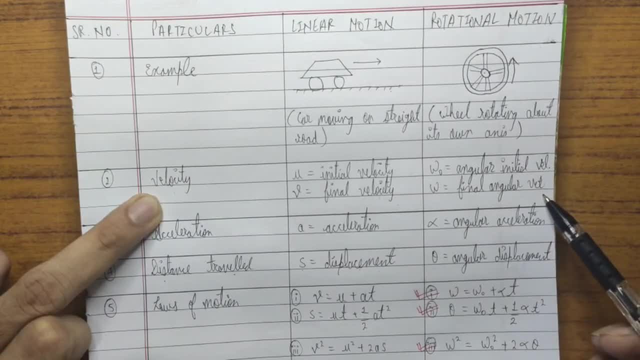 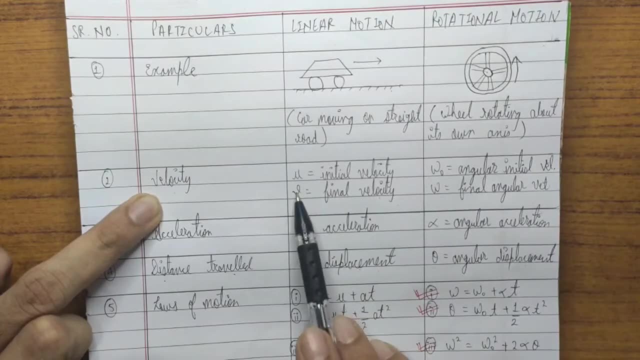 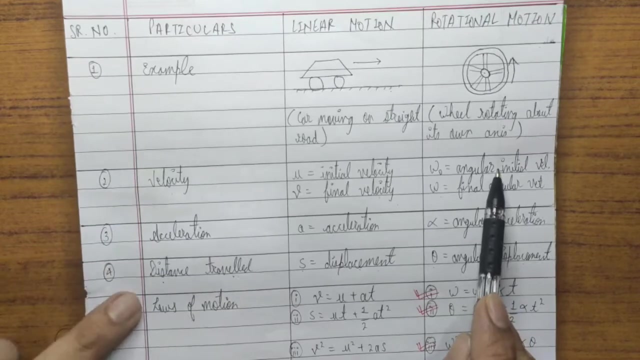 there is omega, which is final angular velocity. okay, so in linear motion it is u and v. in rotational motion it is omega, not and omega. okay, just the notations are different, okay, and in this case it is linear and in this case everything is angular. okay, so we have studied. 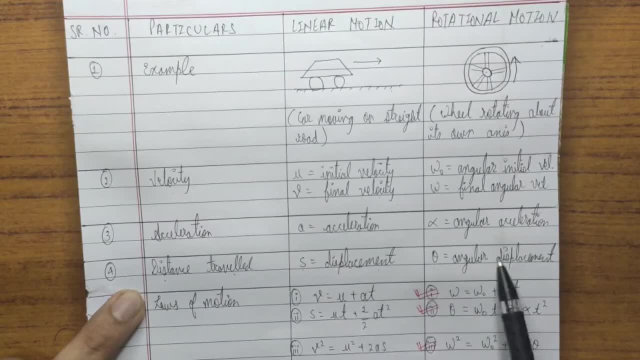 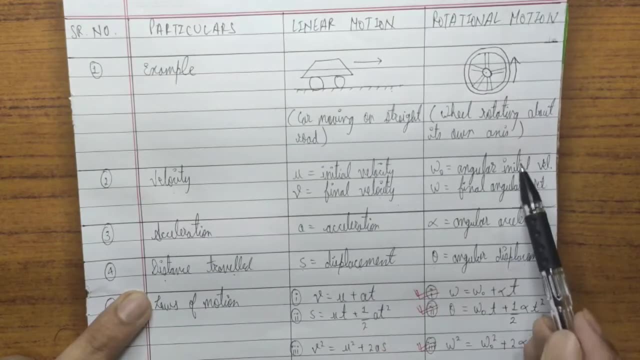 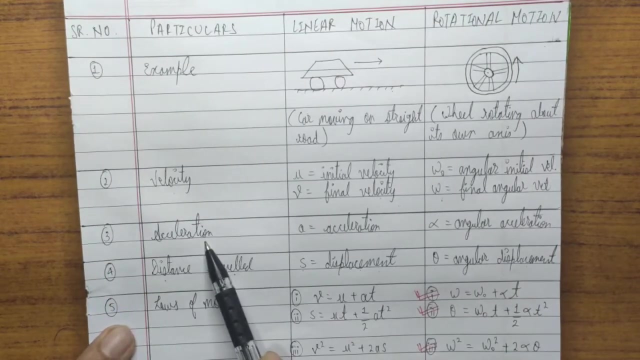 example, we have seen there is displacement and there is angular displacement. we have also seen there is velocity: there is linear velocity and there is angular velocity. initial and final, initial and final, u and v, and in this case omega, not and omega. okay, so now again there is acceleration term. so in linear motion there is linear acceleration, which is: 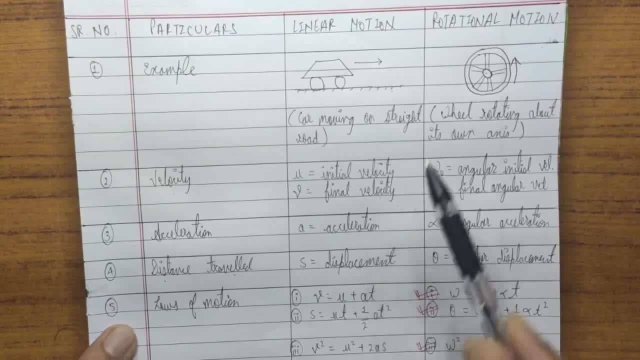 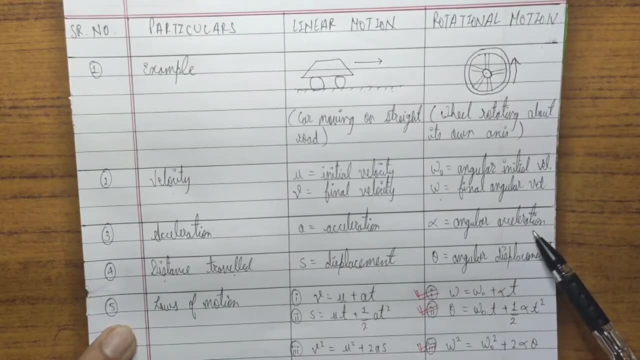 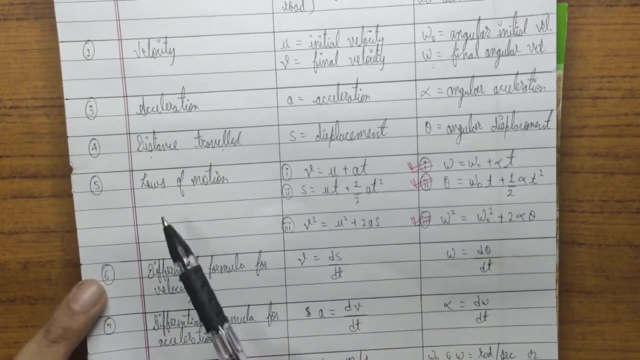 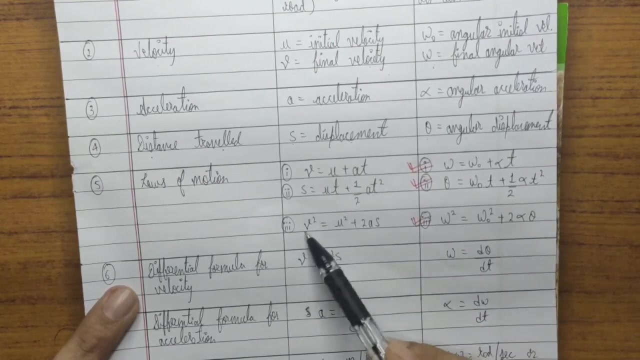 represented by simply a. this is acceleration, which is linear acceleration, but in rotational motion, since we are getting angular velocity, there will be angular acceleration and it is represented by alpha. okay, now moving forward. now we have studied different laws of motion, the formulas, okay. so first is: v is equal to u plus at, s, is equal to ut plus half at square v. 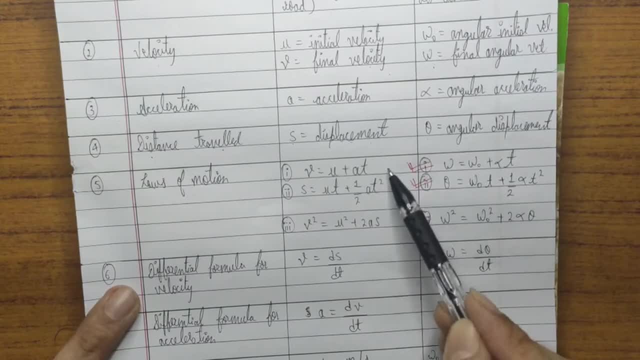 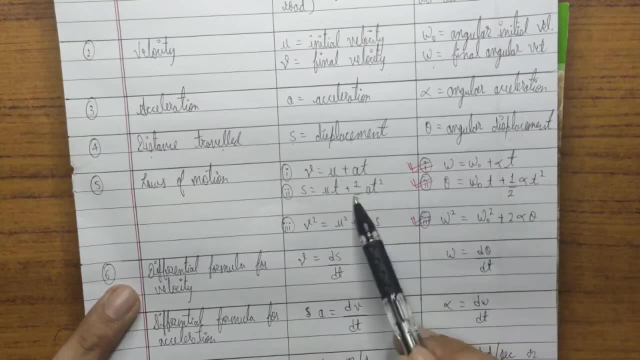 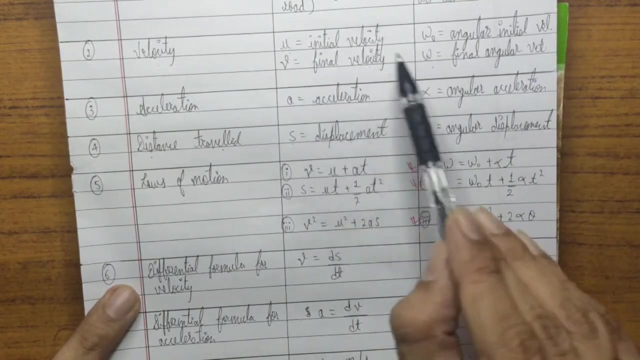 plus twice, as we have learned all these formulas and we have even solved numericals on these formulas. okay, now, in rotational motion, all these nomenclatures are replaced by these terms. okay, so, instead of u, we are putting omega, not instead of v, we are putting omega. instead of a, we are 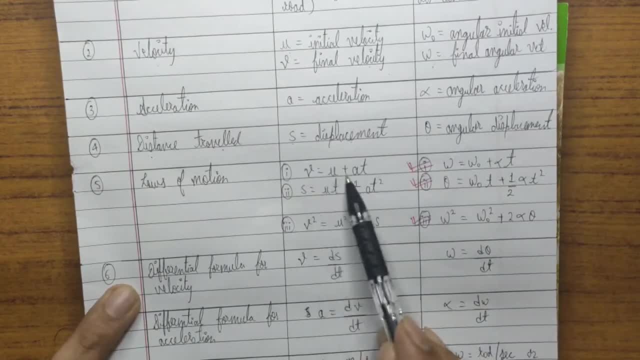 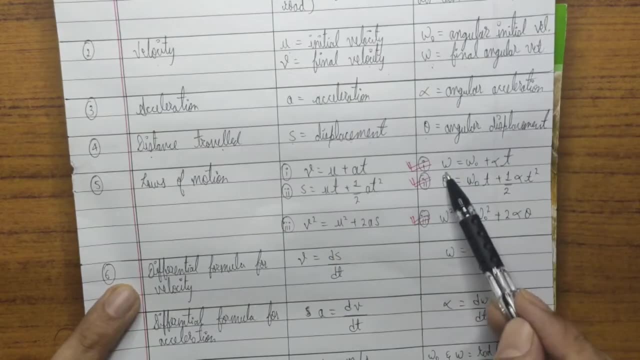 putting alpha and instead of s we are using theta. okay, so first we look at first equation. it is v is equal to u plus at now, what is v, v is nothing but omega in rotational motion. so omega is equal to u is omega not. okay, u is omega not plus. acceleration is alpha, so plus alpha. 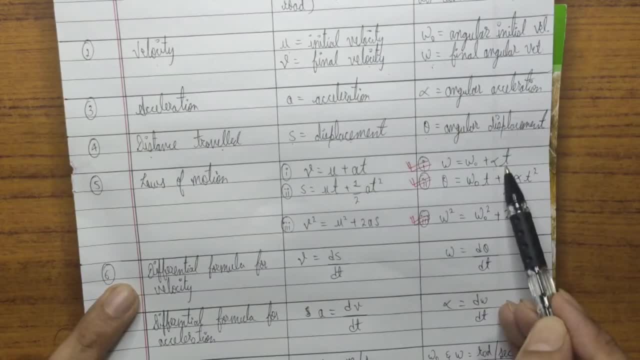 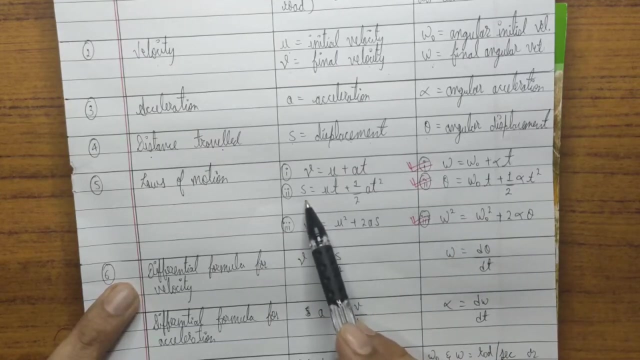 and t will be as it is why? because t is nothing but time. so in linear motion also, the time will be t and in rotational motion also there will be time t. okay, there is no such thing like angular time. okay, time is time itself. okay now, similarly, we have replaced all these terms and we have mentioned 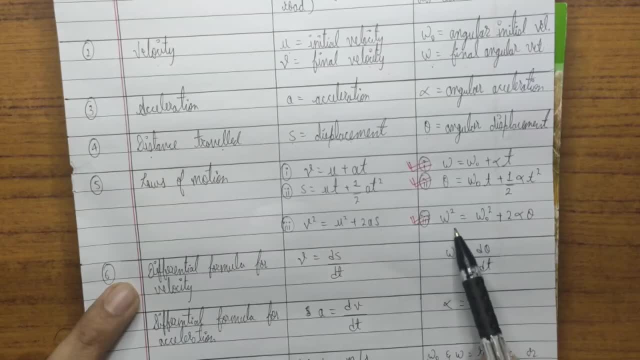 all these terms in this equation and we have come up with this third equation. so in linear motion, there are these three formulas. in rotational motion, there are these three formulas. okay, no need to learn these formulas. if you have learned all these formulas, okay, just you have to replace each term. 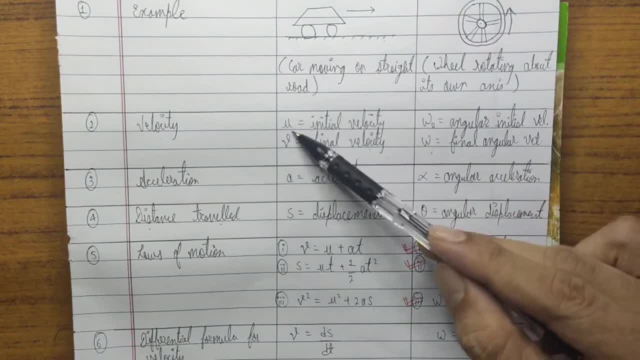 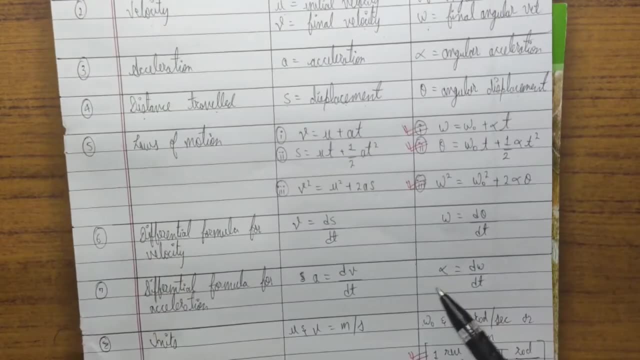 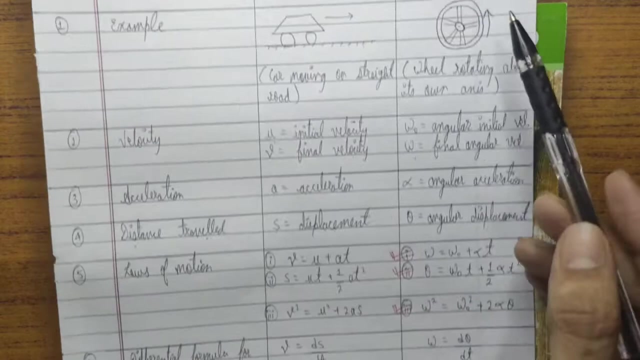 okay, just remember these things. okay, how u is replaced by omega, not v is replaced by omega, a is replaced by alpha and s by theta. okay, so while solving numericals, you will have to use these formulas, not these formulas. okay, for solving numericals on rotational motion. 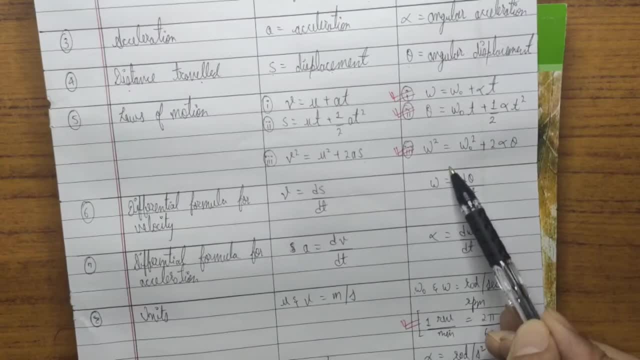 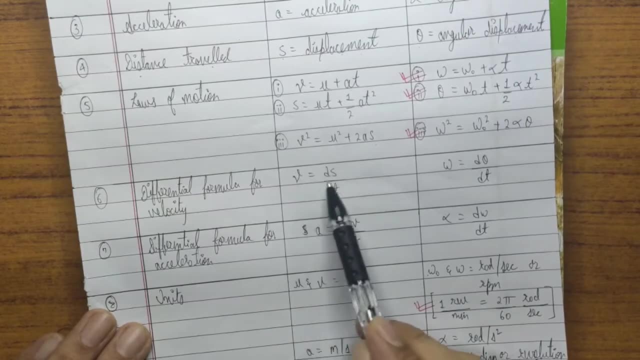 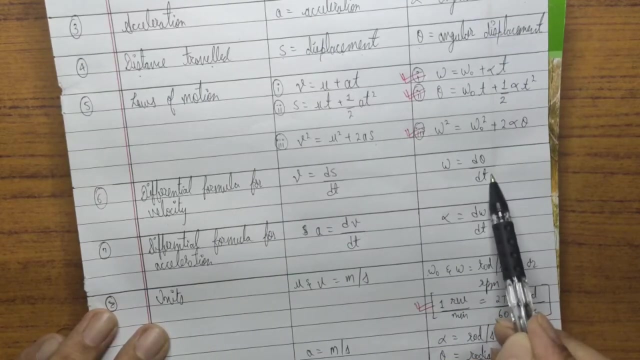 okay, you have to use these formulas. okay, now, differential formula for velocity. okay, we know what is velocity. velocity is nothing but rate of change, of displacement with respect to time in case of linear motion, but in rotational motion. okay, in this case, that is velocity. in this case, 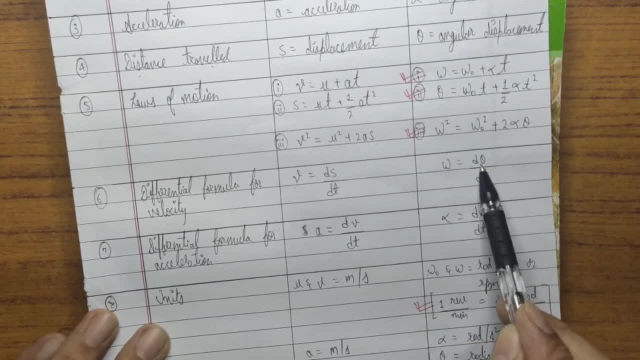 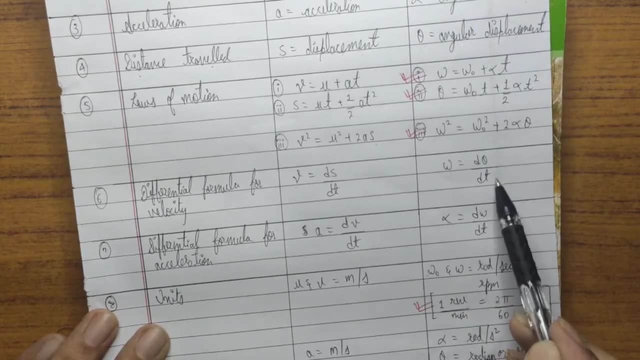 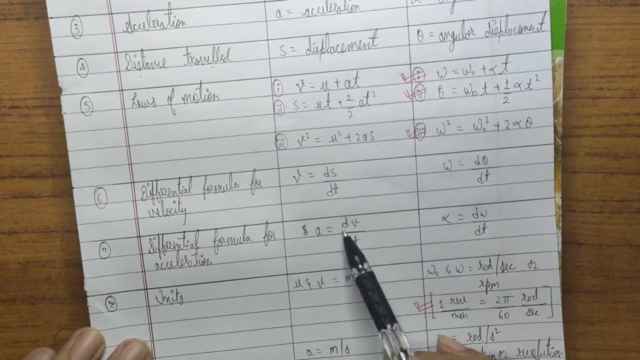 it is angular velocity, so this angular velocity will be change in angular displacement with respect to time. here, change in displacement with respect to time. change in angular displacement with respect to time. now differential formula for acceleration. okay, now, acceleration is what change in velocity with respect to time. but in this case it will be. 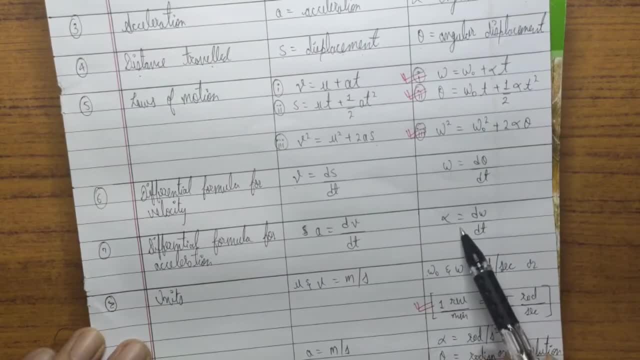 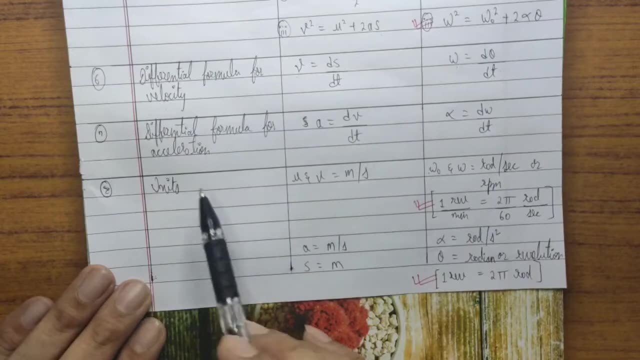 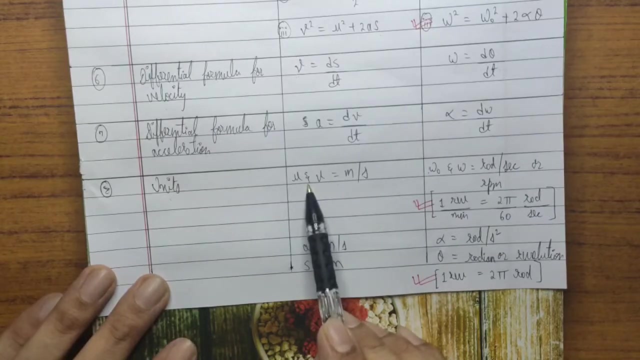 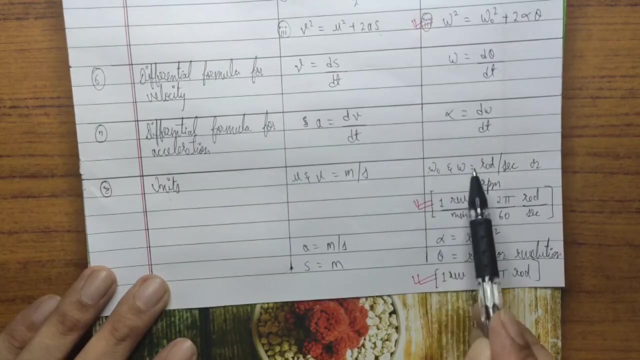 change in angular velocity with respect to time. so alpha is equal to change in angular velocity with respect to time. okay, now last part is units. okay, so in linear motion initial and final velocities are represented, or the units which are used for representing velocity is meter per second. okay, but in this case the velocity is angular. okay, 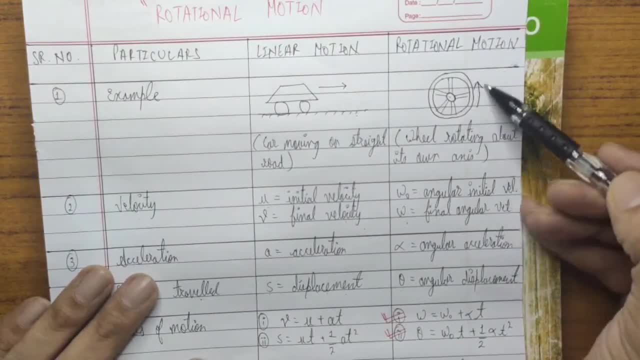 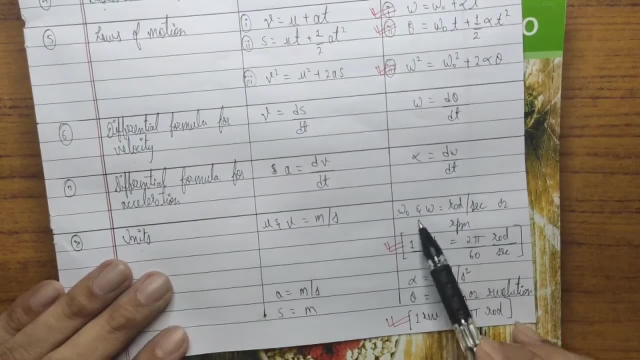 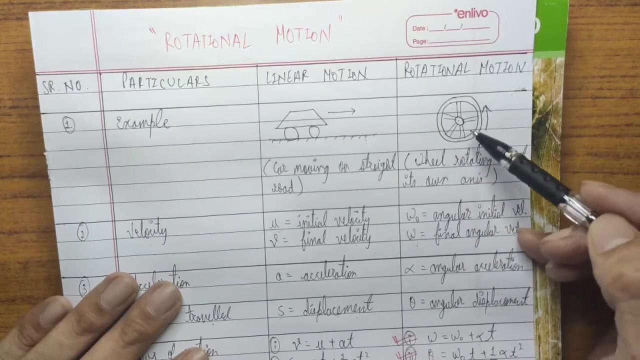 this wheel, it is rotating by a certain angular velocity. okay, by a certain angle, so the unit will be radian per second or revolutions per minute. okay, this wheel, since it is rotating, so we can calculate the velocity by calculating what will be the revolutions per minute. so suppose, 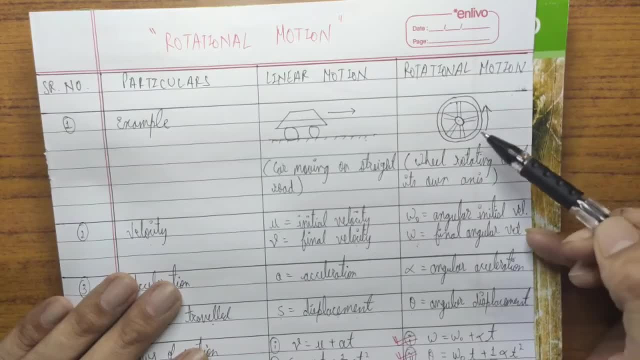 i say this wheel is rotating by 100 revolutions per minute. that means in one minute this wheel is rotating 100 times. so that is nothing but the velocity revolutions per minute. or we can say it is radian per second. so by suppose i am saying that this the velocity of this wheel is, say, 100 radian. 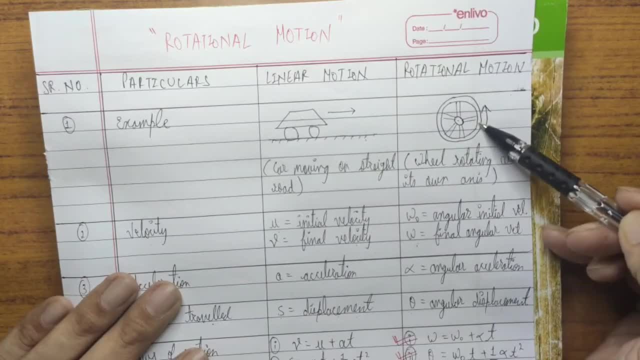 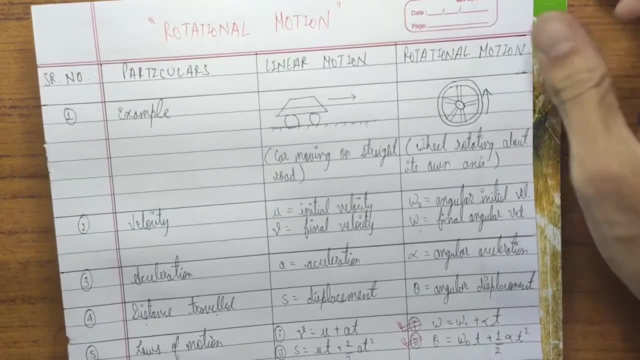 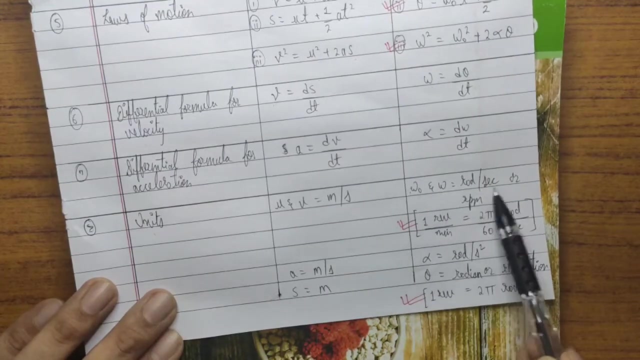 per second. that means that this wheel is turning 100 revolution, 100 radians, that is angle, 100 radian per second. okay, so that is the unit for velocity. so remember this unit. this is very important. okay, so the velocity may be represented in radian per second or rpm. okay, and since there, 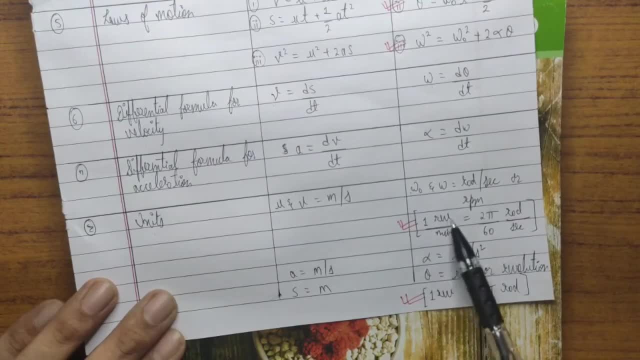 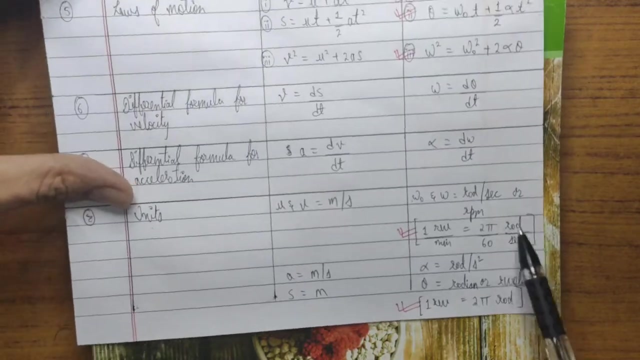 are two units. you need to understand the conversion. okay, so 1 revolution per minute, or 1 rpm, is equal to 2 pi upon 60 radian per second. okay, you have to remember this. this is very important while solving numericals. okay, many times the velocity is given in rpm and you have to convert it it into radian per second. so, okay, so, 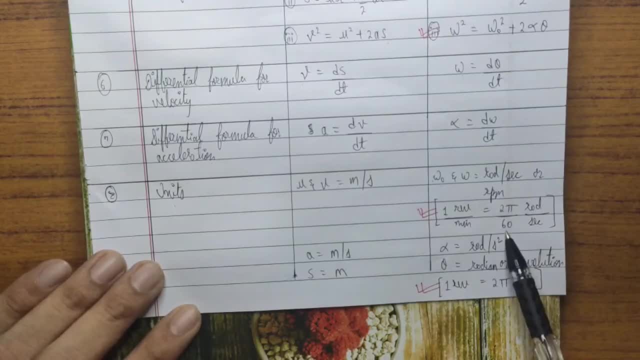 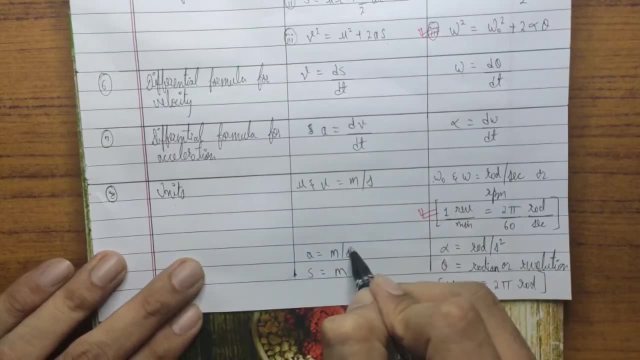 for converting, you have to multiply by 2 pi upon 60. okay, now in this case its acceleration. we know what is the unit for acceleration: it is meter per second square, okay. it is not meter per second. it is meter per second square, okay. and in this case, instead of acceleration, it is angular acceleration. 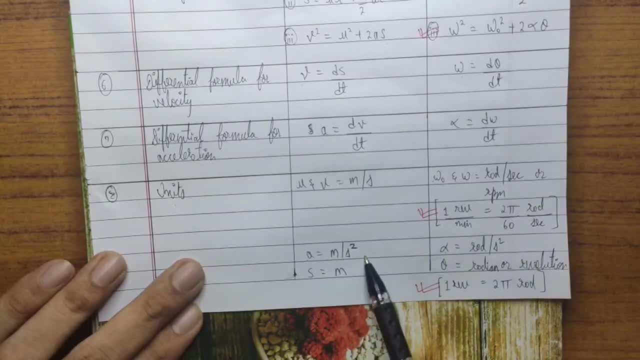 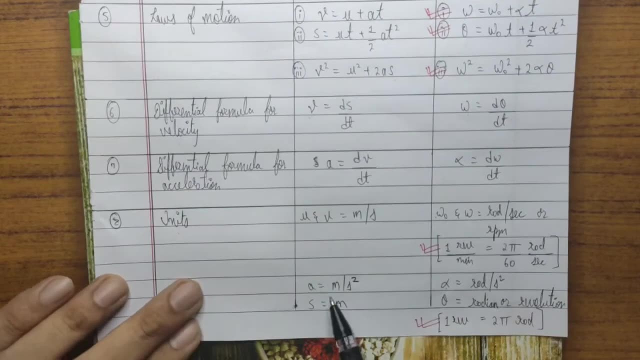 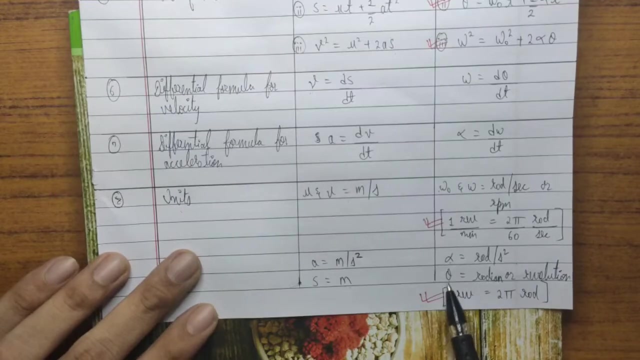 which is represented by alpha and unit will be here. it is meter per second square, here it is radian per second square. so if you see, the meter is replaced by replaced by radian, okay. so meter per second square, it is radian per second square, okay, and displacement is meter and in this case it is. 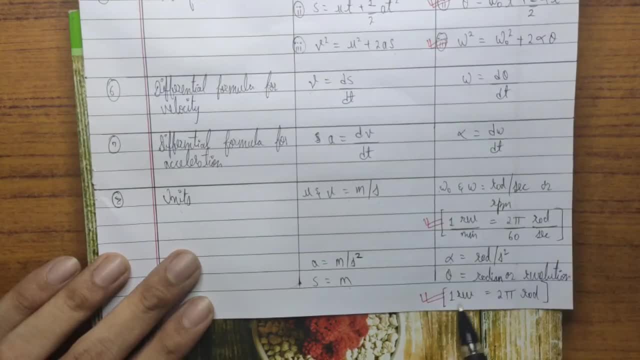 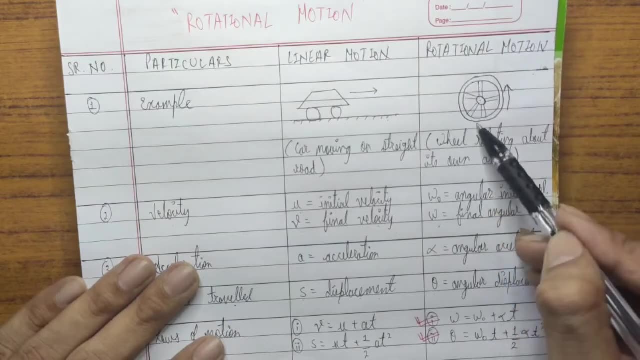 angular displacement, which is radian or revolution. okay, and again, 1 revolution is equal to 2 pi radian. right see 1 revolution, the 1 revolution of wheel. that means the wheel is rotating by 360 degree. and what is 360 degree? it is 2 pi. so that is why it is given.